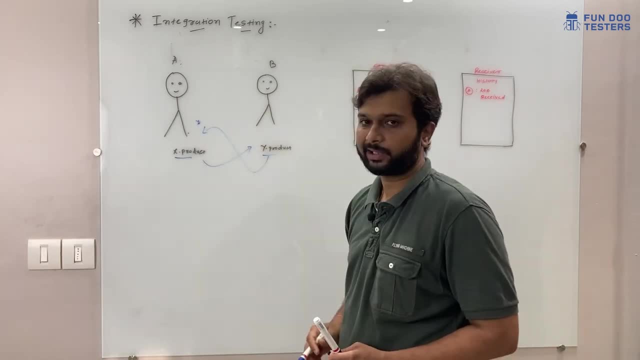 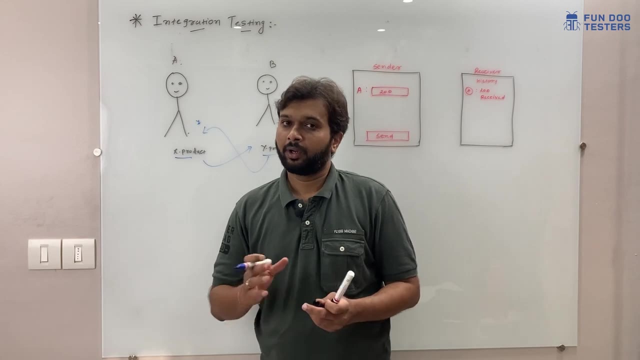 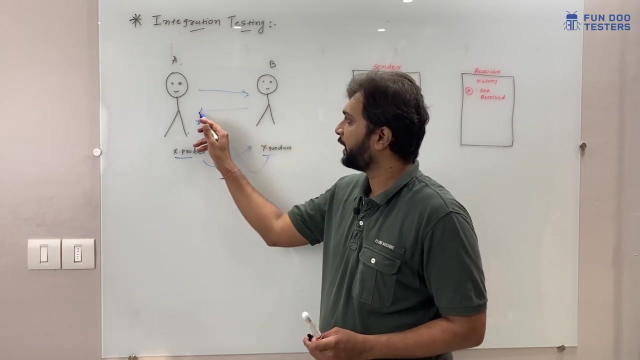 they will give few quantity of Y product to person A. So this is how they used to make a transaction when there was no currency. In the similar way, when module A sends data to module B and module B sends back some data to module A, that is called integration testing. 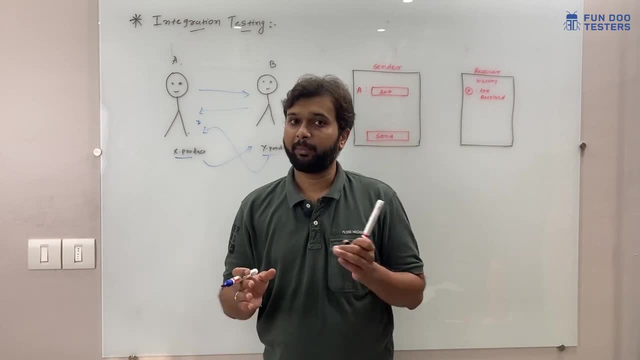 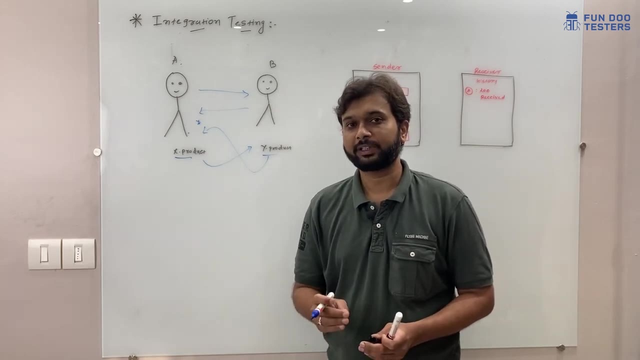 So testing data flow between the module A and module B, or testing the data flow between two modules- that is called integration testing. So in this video we are going to understand what is integration testing, How we can perform the integration testing, What are the types of integration testing. 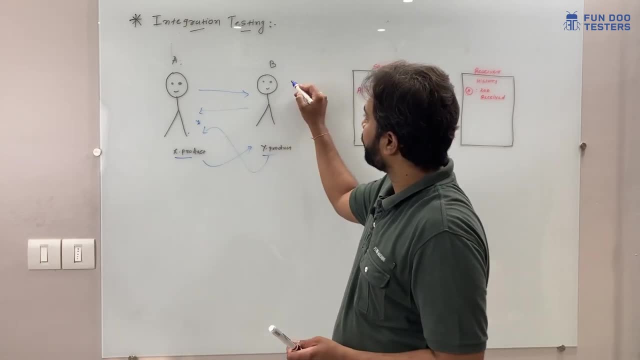 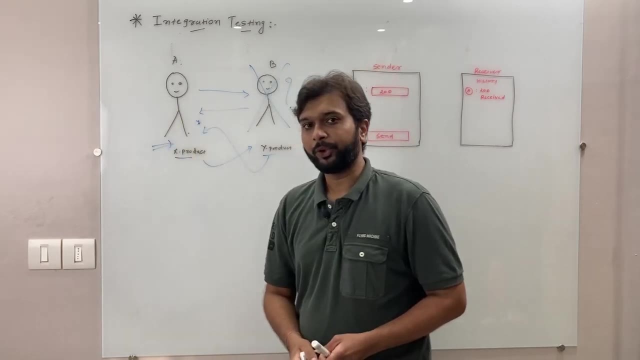 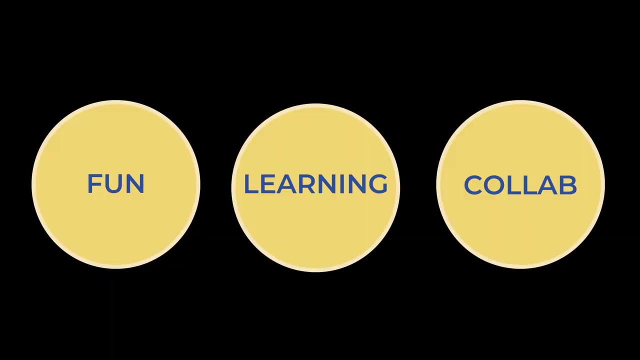 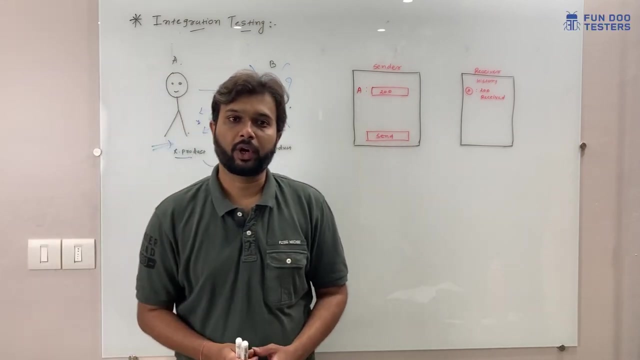 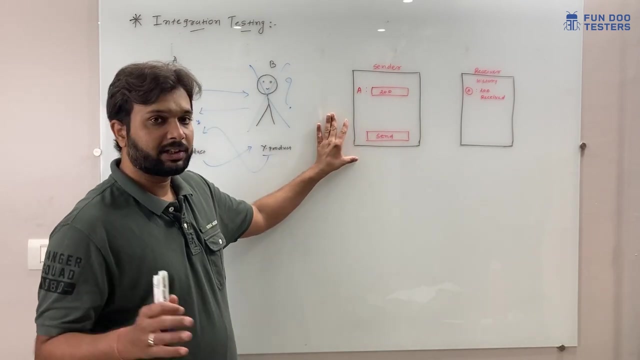 and very important is, for example, person B is not exist, Then how we can test a module after a small interval. So let's take a real time example. Nowadays we all are using wallet or we are sending data online from person A to person B. This is a simple screen. 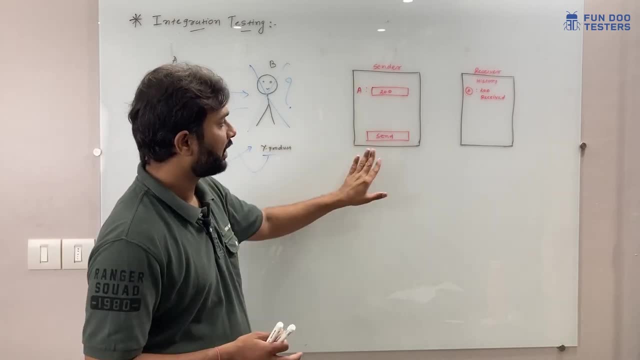 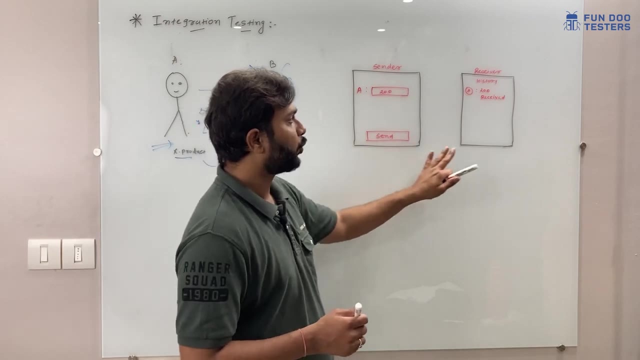 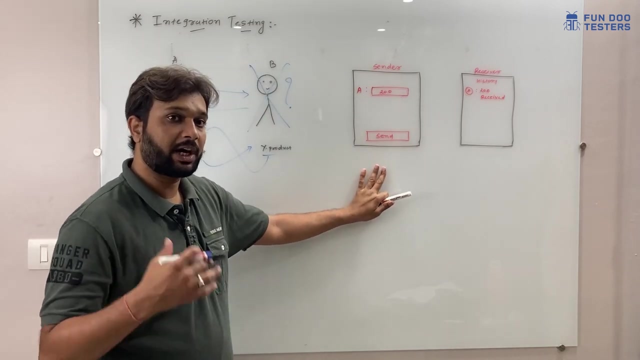 of wallet application. First one is sender screen and another is receiver screen. Let's say person, A sender wants to send 200 bucks to the receiver. So we will understand this scenario and we will understand how we can perform integration testing in this case. 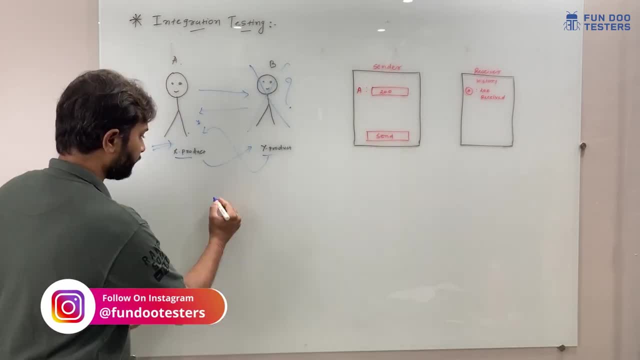 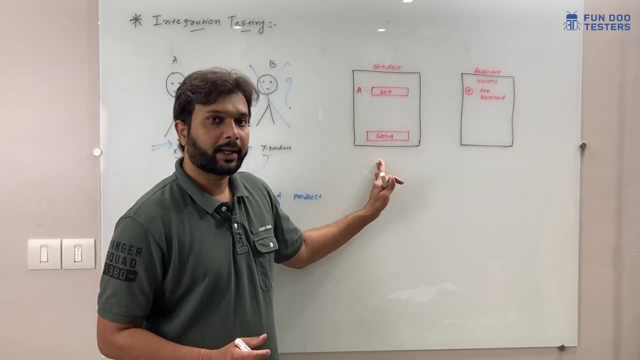 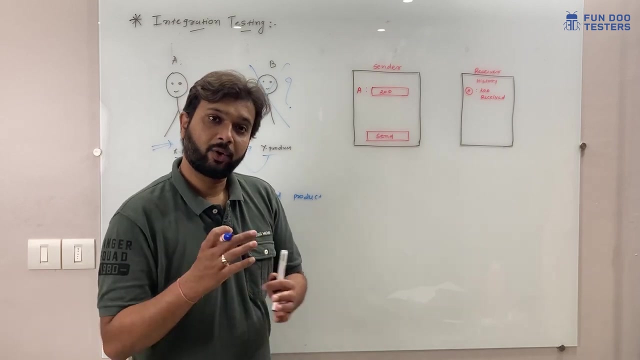 So initially we have to understand the product. Our first scenario is: understand the product. Here we are going to test the online banking application. Once online banking comes in our mind, we are going to send money or transaction related things. we are going to test, Right. 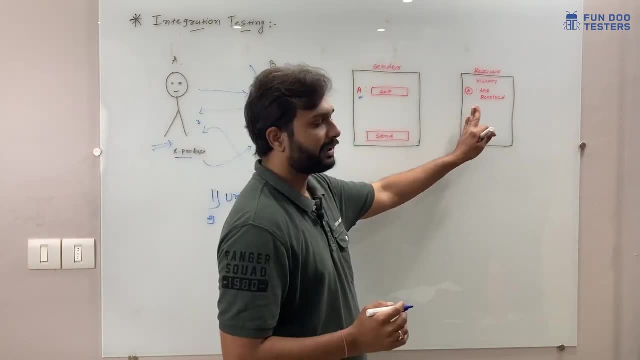 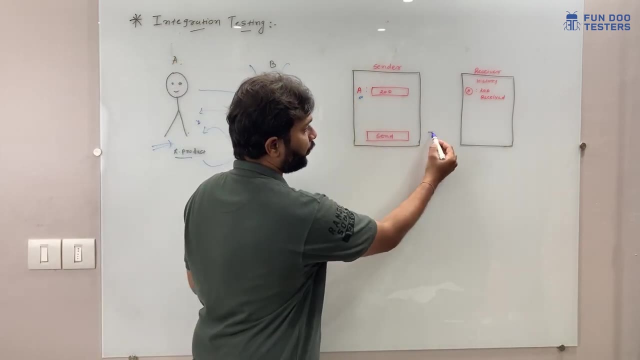 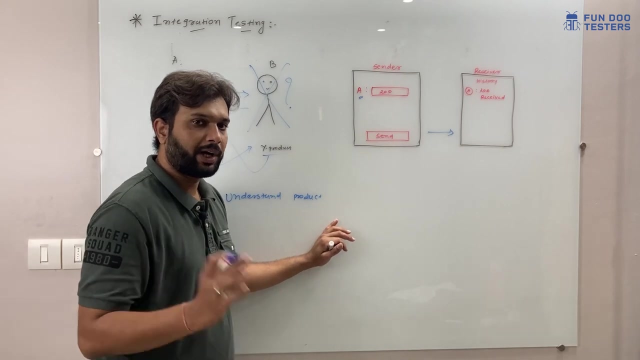 Yes, So here this is the amount screen and this is the history Amount. is user A or sender is sending 200 bucks to user b, so user will receive the amount and in history section we can see the transaction detail. this is the normal scenario. now we have to break down all the 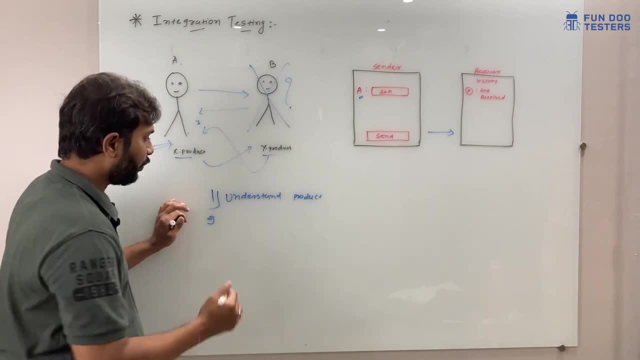 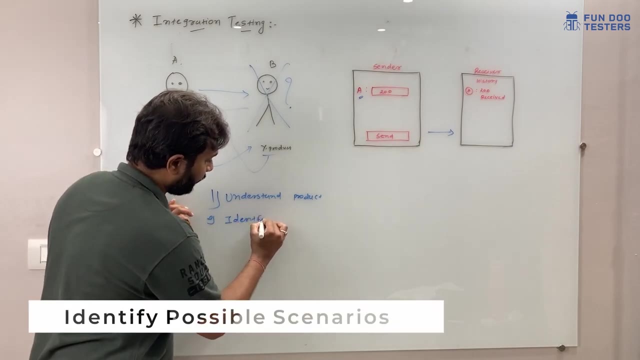 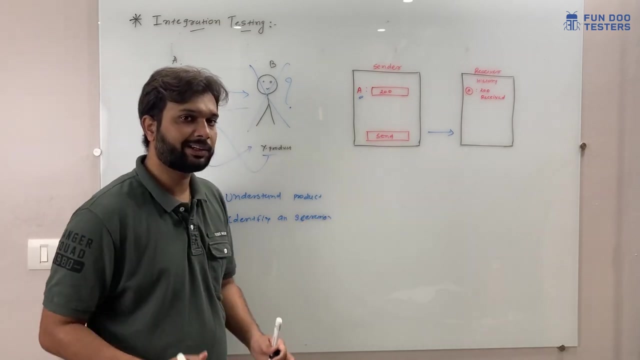 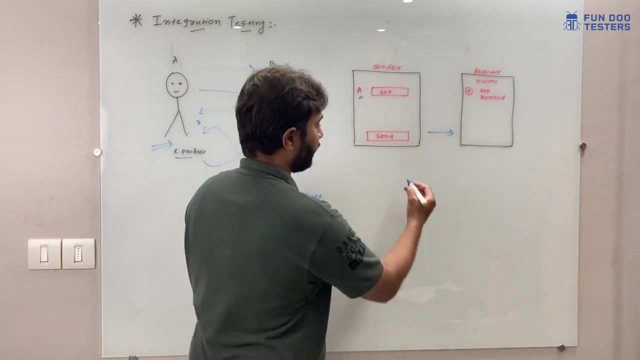 scenarios we once we understand the product. later on we have to prioritize or identify all possible scenario. so later on, identify old scenarios. so here, what are the scenarios we can make? so first is receiver s2 available on the wallet let. next scenario is we have to link our bank account. 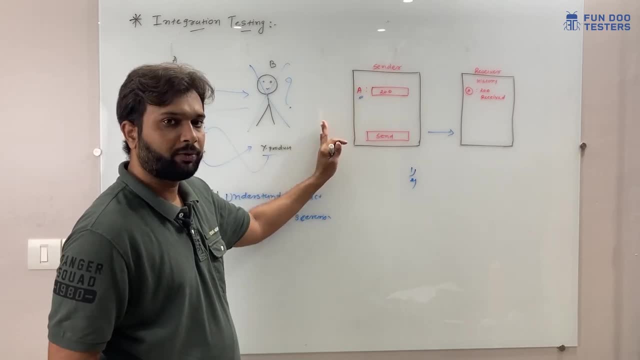 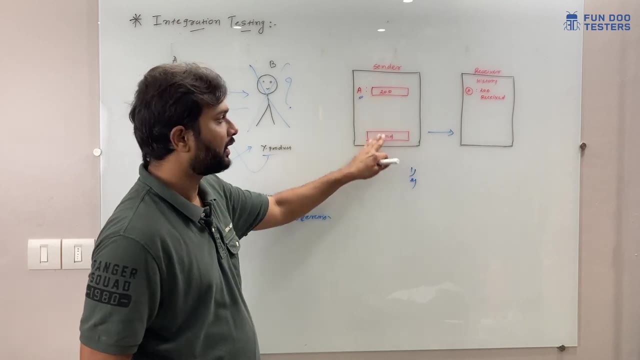 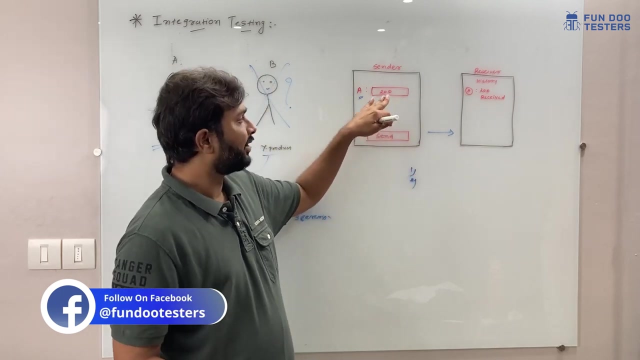 with the wallet application. another is we have to enter the valid data. so if we are not going to enter the amount or we are leaving this field empty, then we can not perform the transaction otherwise. for another scenario is if person b is not available, we are trying to look, look, look at. 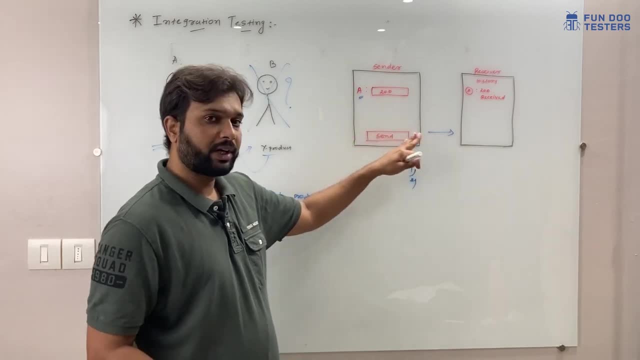 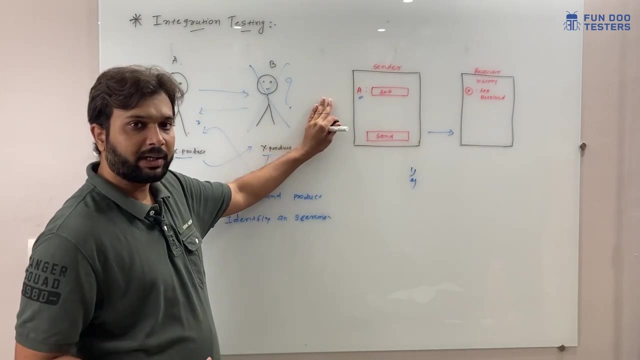 for this person and that person is not available, then we cannot perform the transaction. we cannot test the integration scenario later on. if we have added invalid bank details before that, we are going to add the bank details. if we have credit card or debit card, we are going to store the data. 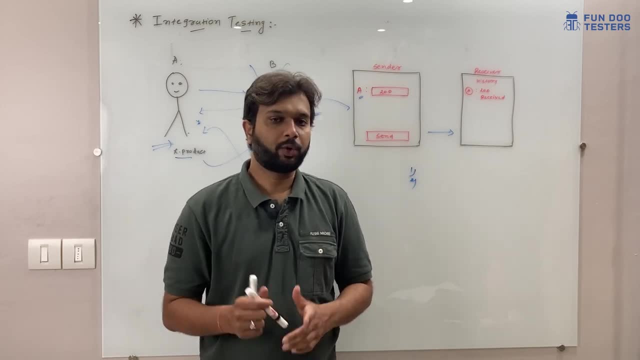 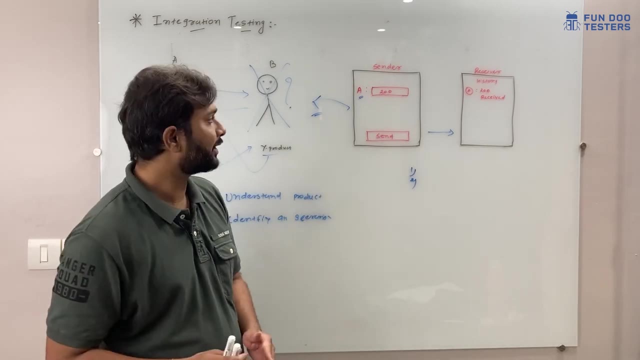 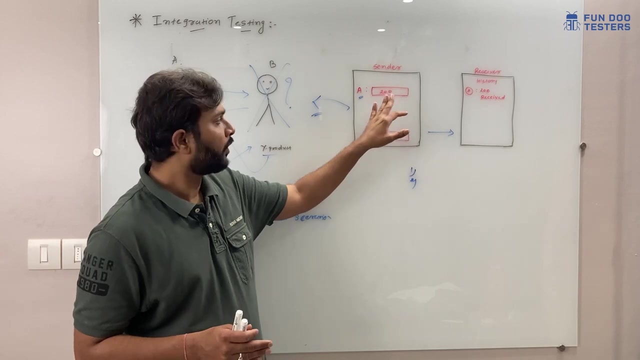 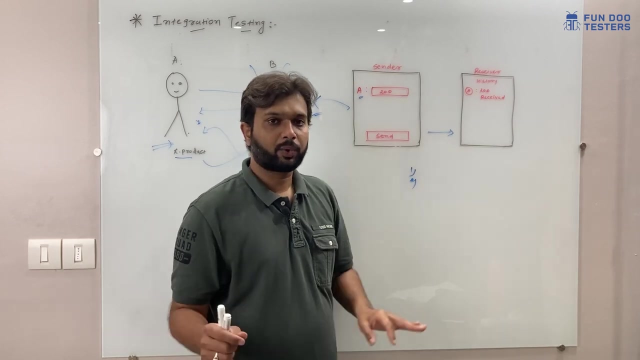 we have to generate the pin. so if we have not performed prior steps, then we can not perform the transaction later on. for example, we have to perform few functional scenarios like entering invalid amount, leaving this field empty, and we have to try to send the amount. so if you are not aware about, or if you are not aware of functional testing, then please go to the. 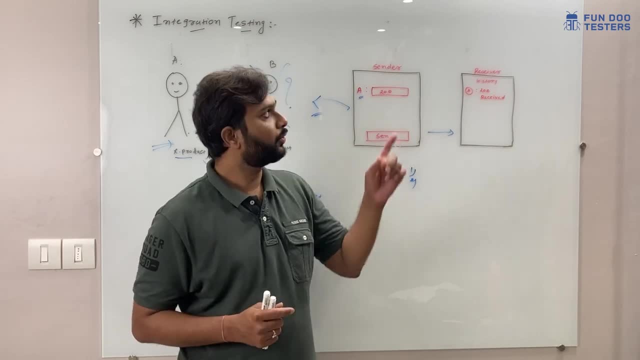 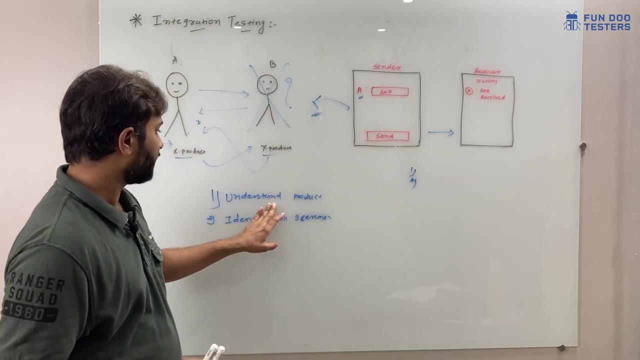 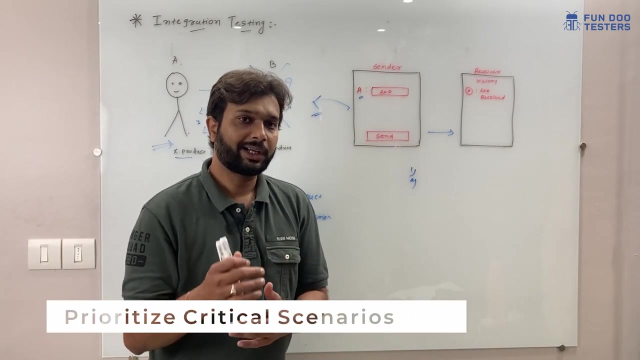 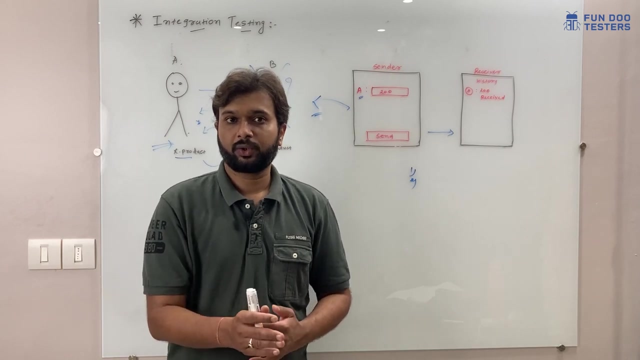 description section and you can find a video of functional testing or you can go from the card. so these all are the scenarios. now we understand the scenarios. we have identified all the scenarios. later on we have to prioritize scenarios because in the real time first we are going to test happy flow or real scenario. later on we will jump to the negative scenarios. but 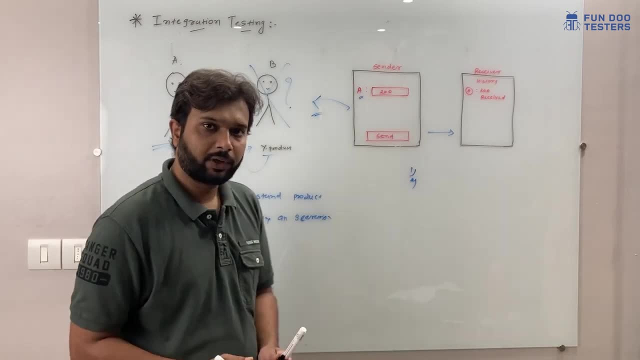 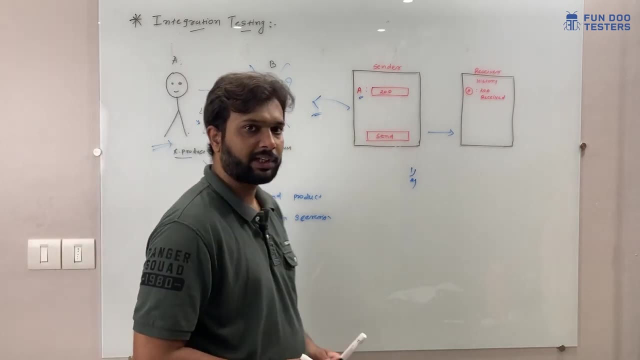 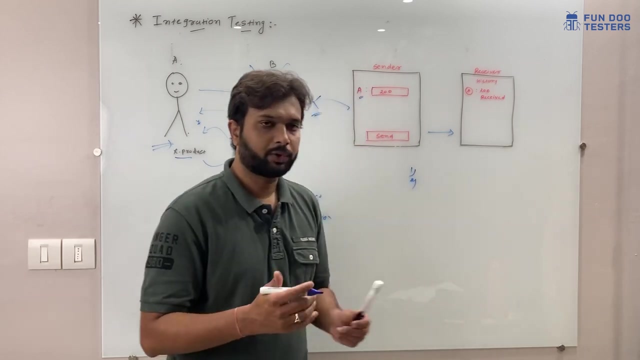 initially we are going to test the happy. first we have to prioritize all the scenarios. first we have to implement a new scenario and after that we are going to test all the scenarios. so once we have prioritized all the scenarios, later on we have to document all the scenarios. 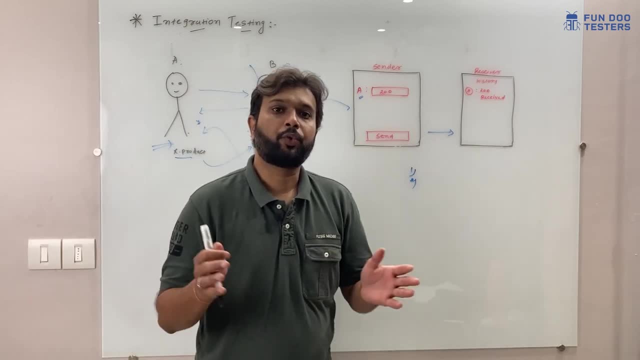 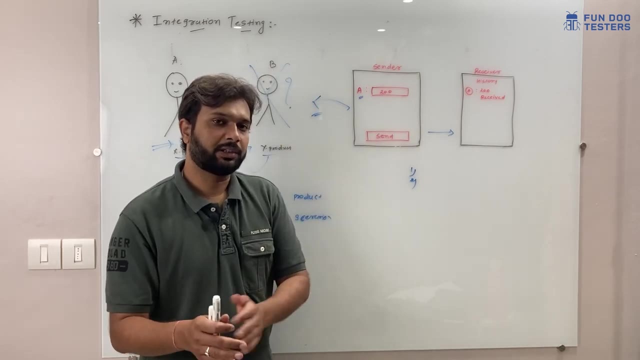 because, for example, i am working on a module, so this is the small application, but in real time we are working on a huge applications. there has to be a proper documentation. let's say i'm working on this applications and after a few months or after two months, i'm going to leave a. 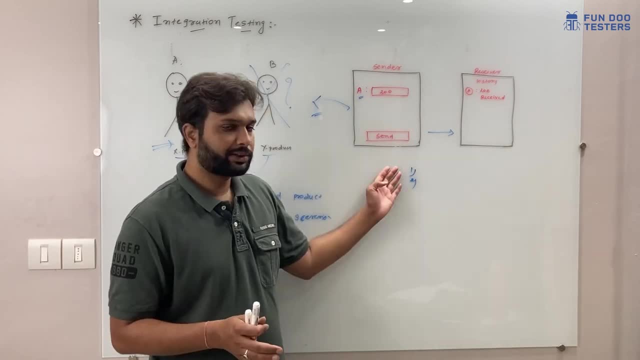 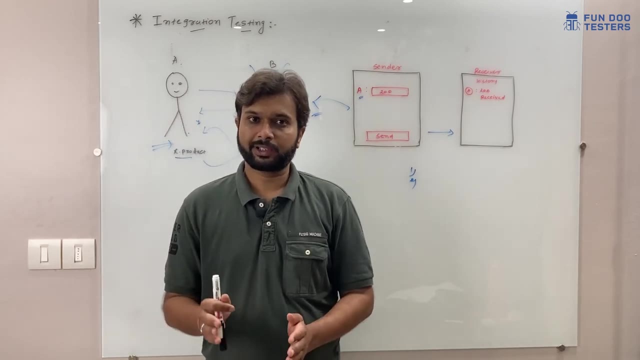 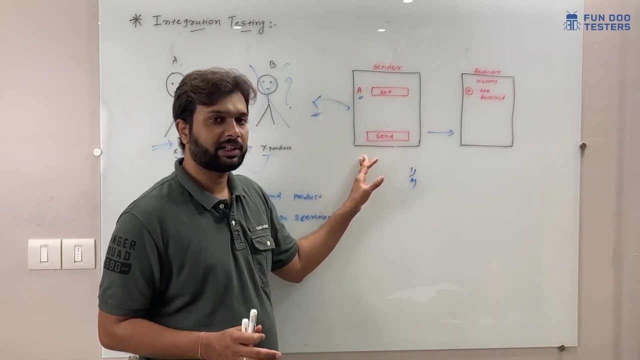 a replacement of me and he or she is going to test on this application. So if there are no document, then he or she has to start from the scratch. If documents are available, then they can go with the document and new guy can easily understand the product. So important is we have to document. 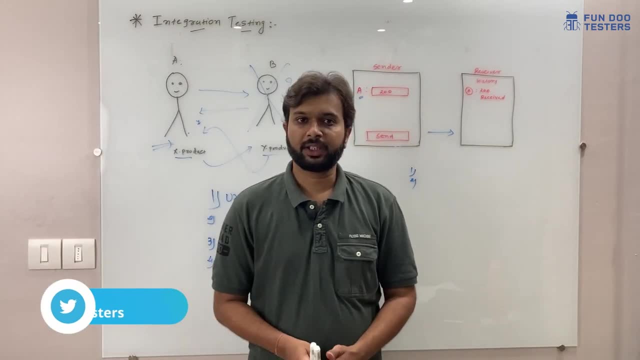 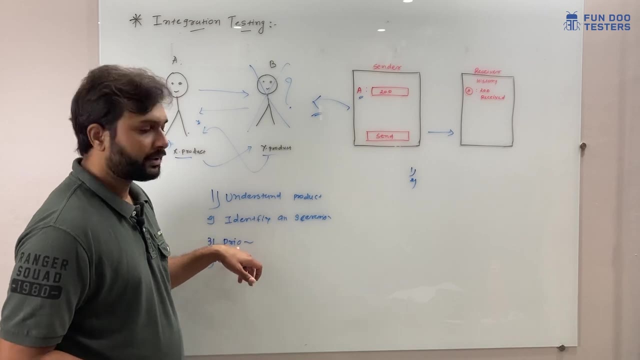 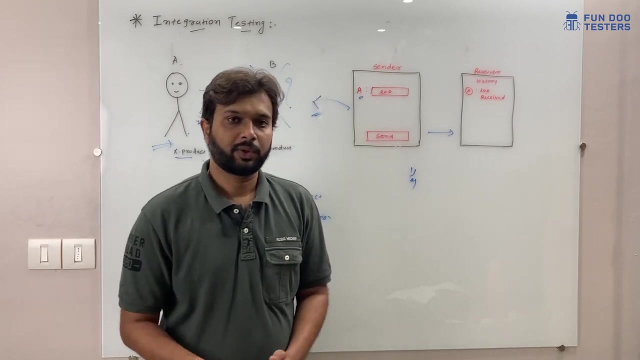 each and everything. and next, in the testing phase, we have to perform. whatever the scenarios we have identified, we have prioritized, we have documented, we have to execute all the scenarios one by one in the testing cycle. So this is how integration testing takes place. Now we will. 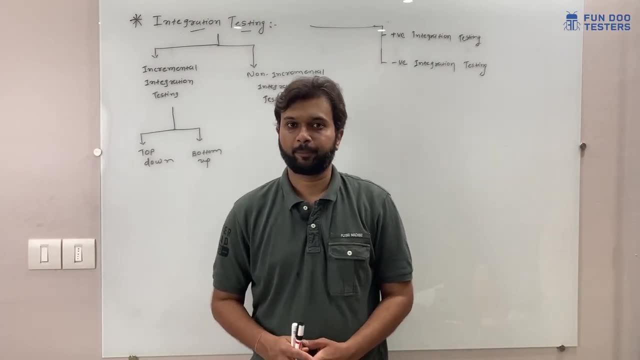 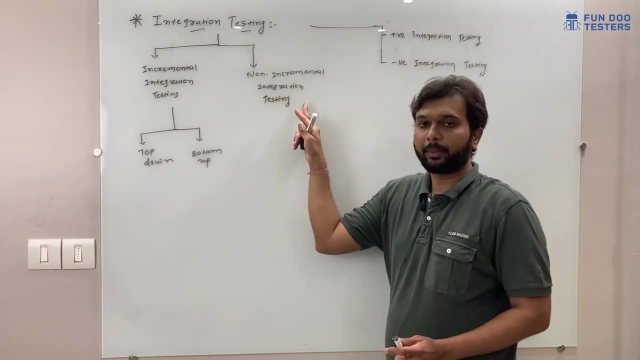 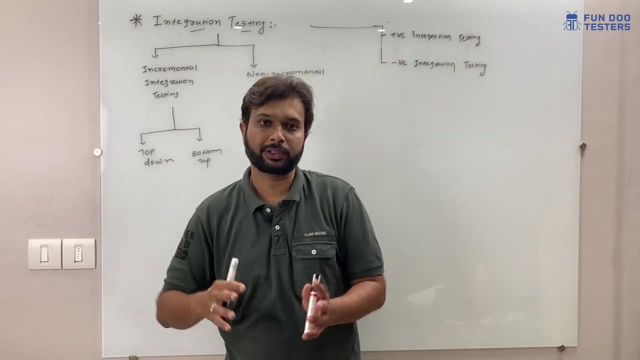 understand different types of integration testing. We can categorize in two ways: One is incremental integration testing and another is non-incremental integration testing. So let's break it down. So when we have multiple modules and we can identify which module comes first, 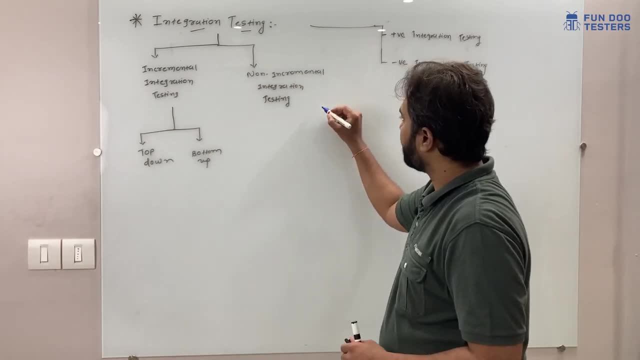 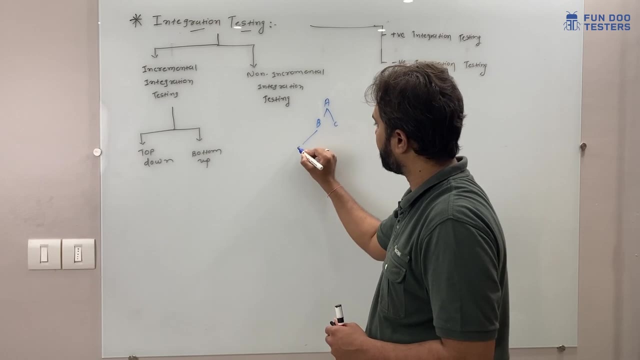 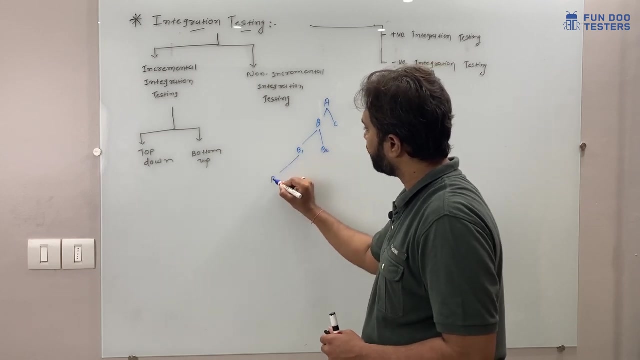 So, for example, in real time we can have multiple modules. so application start with the A, then here we can have B and C, Here we can have C, D, we can have B1, B2, B11,, B12,, B13,. 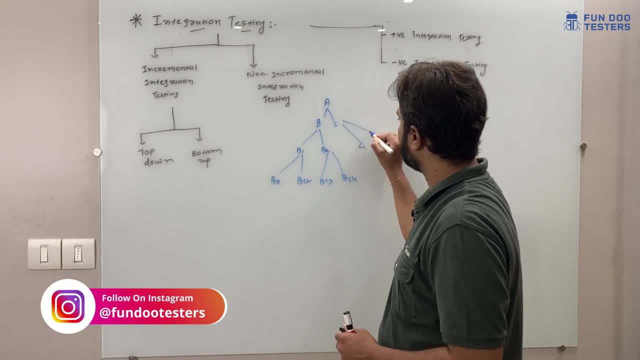 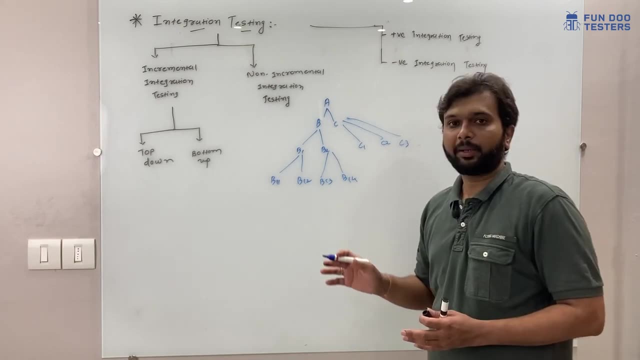 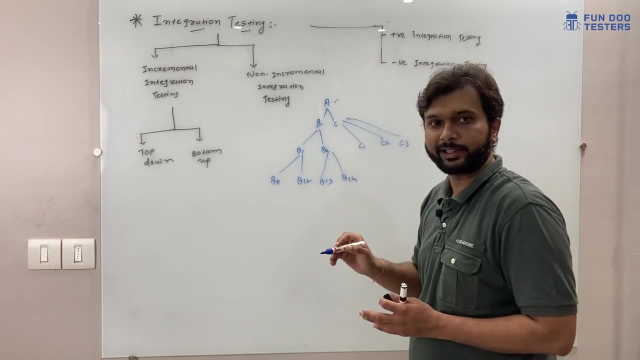 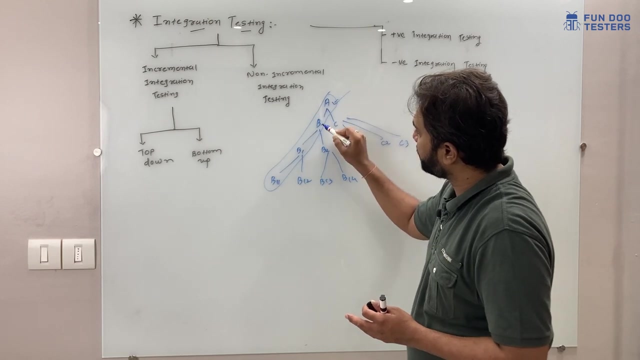 C14, C1, C2, C3. Like this, we can have multiple modules in hierarchy, Incremental integration, testing what will happen. we have to identify which module is parent and which module is child. In this case we. it is starting from the A. A is coming first, now B, B1 and B11.. We can write it. 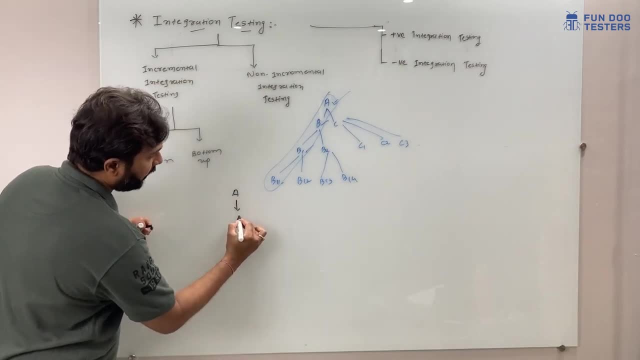 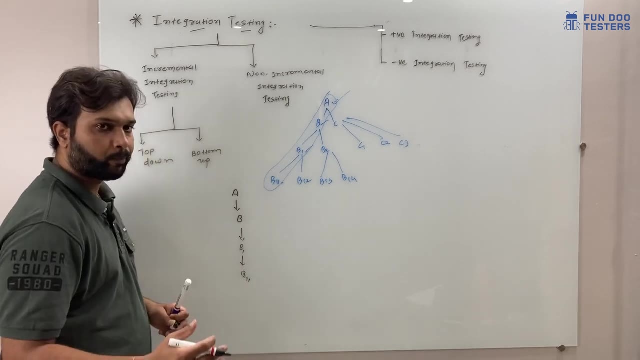 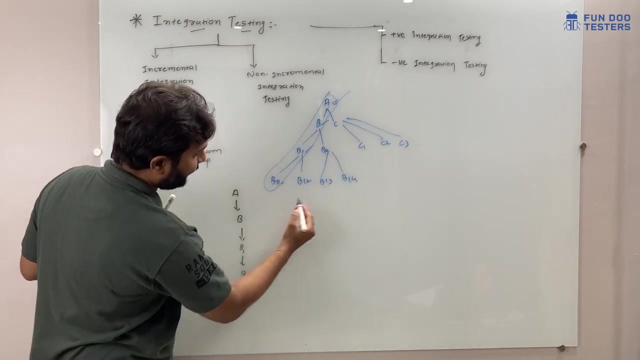 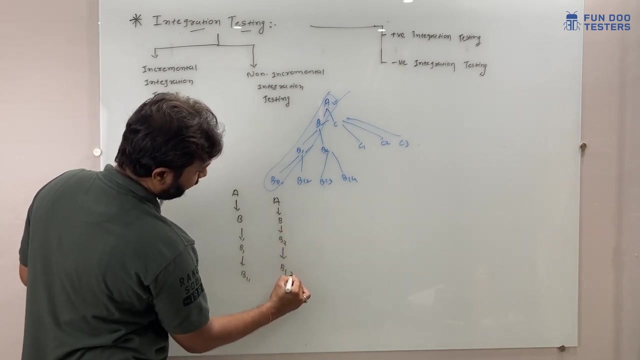 from A to B. It is starting from A to B to B1 and B11.. Another is A, B, B2 and B13.. A, B, B2, and B13.. This is the first cycle and this is another cycle. to test integration flow between the A and B, B and C, B and B1 and B and B11.. In this flow we have to test A and B, B and B2, B2 and B13.. We have to test integration between: 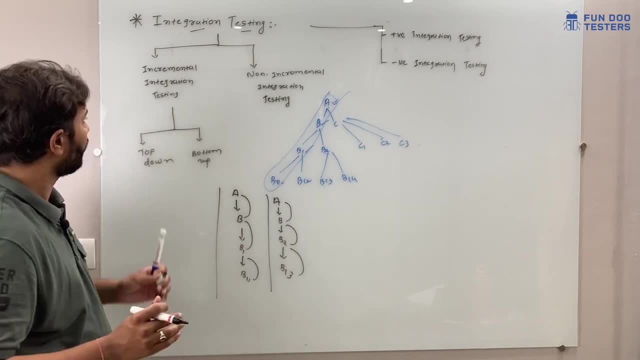 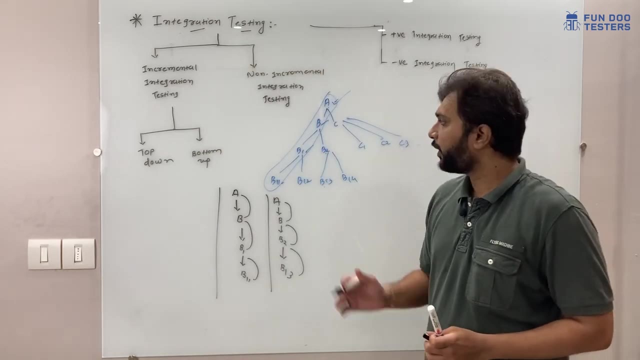 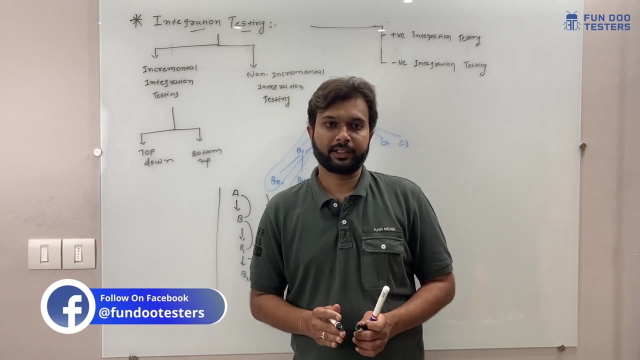 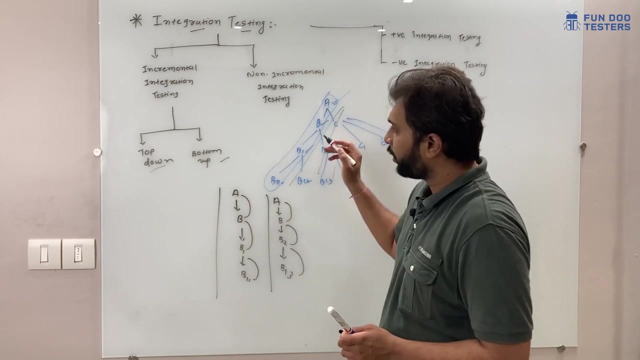 the all these modules And when we can do the incremental integration testing, whenever we are able to identify the hierarchy of the integration. in that case we can perform the incremental integration testing. Now there are also two parts. One is top down approach and another is bottom up approach. We understand the hierarchy. Now we can say that this is 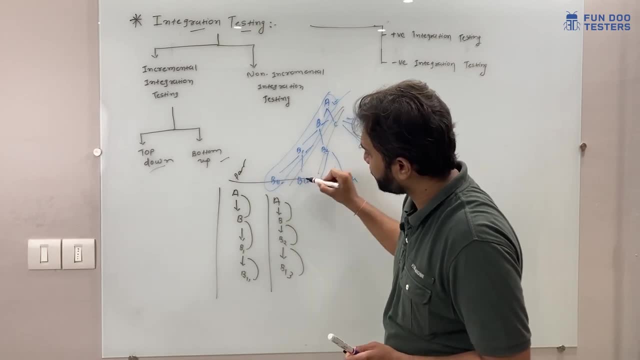 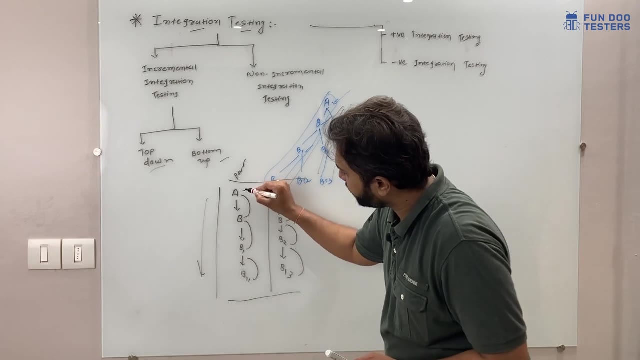 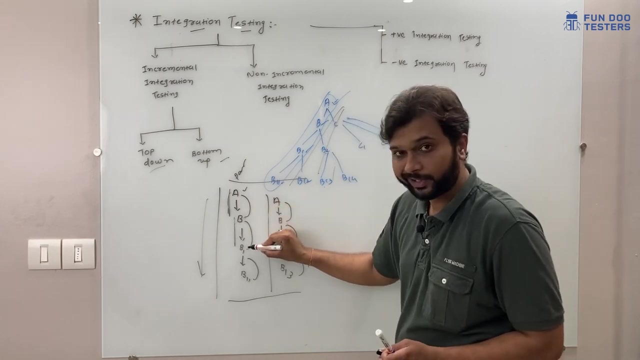 my parent module. This is starting from the parent module and we can go down. If we can go down, these all are our child modules. So A is a parent module In the first phase. A is a parent. B is a child. In this phase, B is a parent. B1 is: 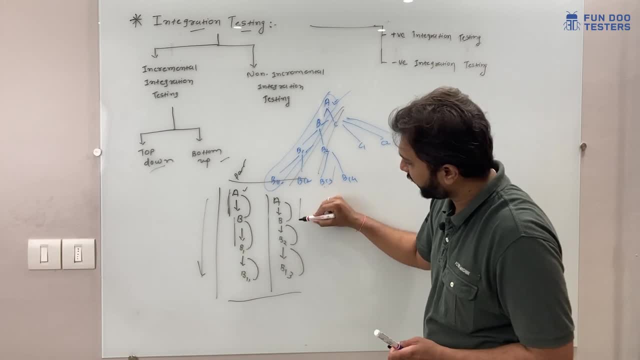 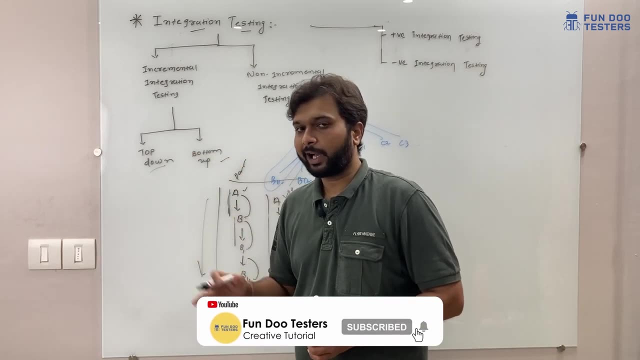 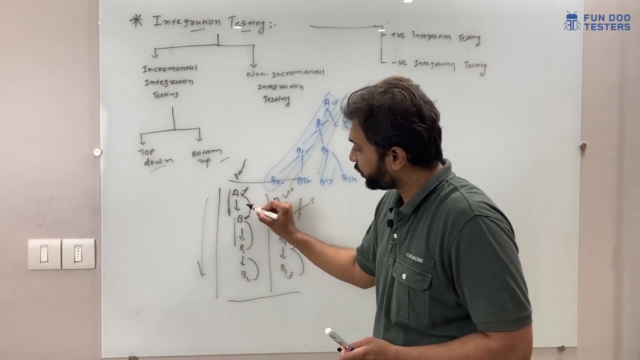 a child. If we take example here, then A is a parent, B is a child. So in top down approach we have to start with the top. We have to start with the A module and then we can go with the B. So we have to test data flow between the A and B. That is called top down approach. 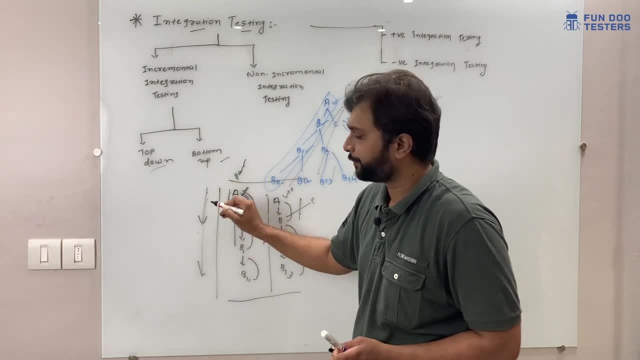 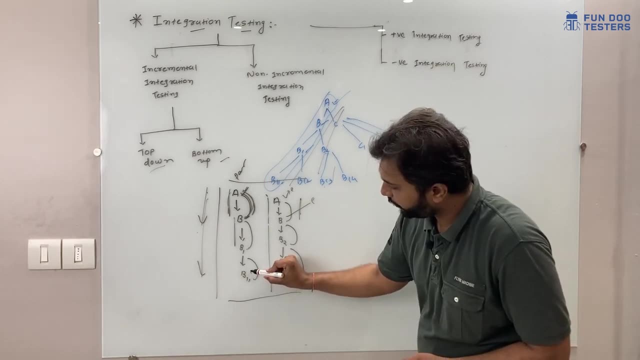 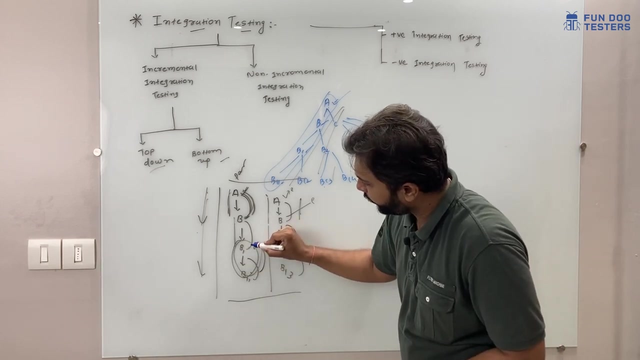 We are going from parents to child In bottom up approach. we have to go to the reverse. We have to start from the B11.. We are going to B1.. First we are going to check integration between these two flow. Later on we'll move to the from B1 to B. We will test the integration between. 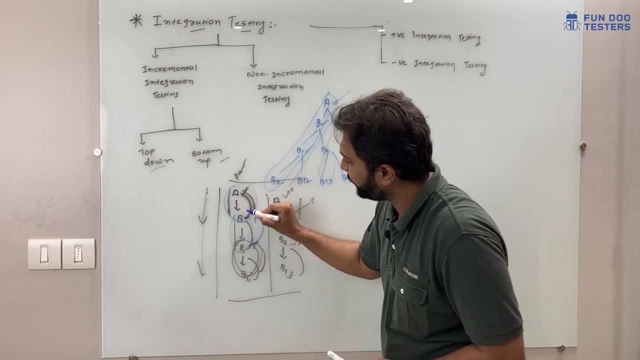 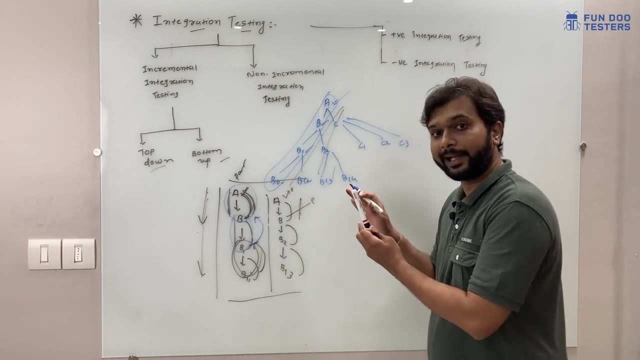 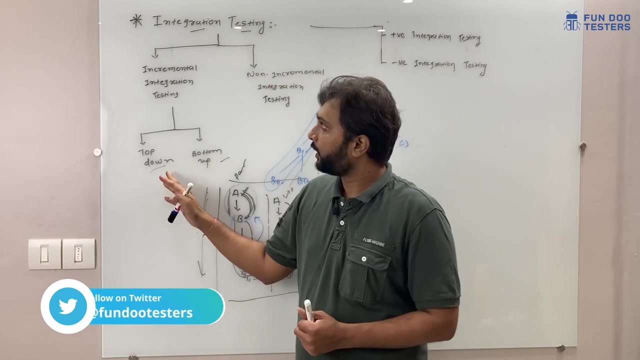 B1 and B And later on we'll move to B2A. We are moving towards parents from child, So that is called bottom approach, Bottom up incremental integration testing. Now what is the advantages and disadvantages of these two? In top down incremental integration testing, we are going from the top to down. 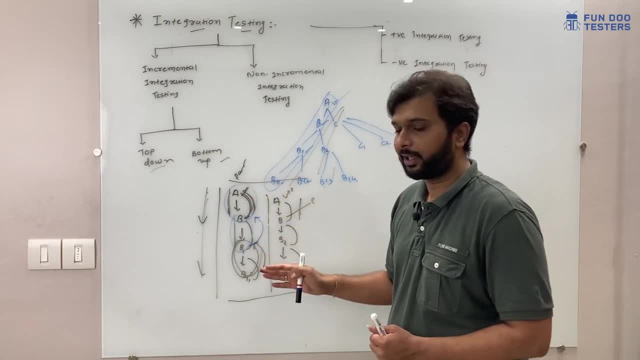 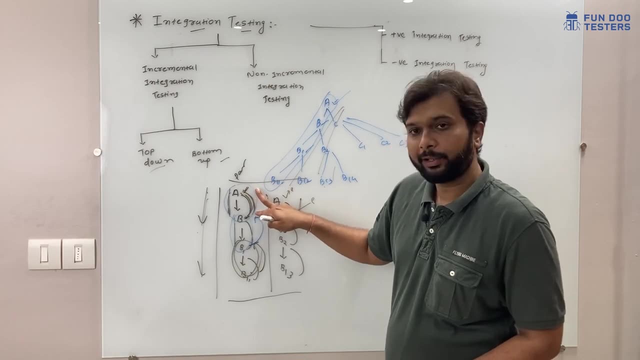 In this case, we have each and every module ready. Why? Because we have created entire hierarchy And whenever we are going to test A module, by that time only we need B module. We are not going to worry about the B or B. 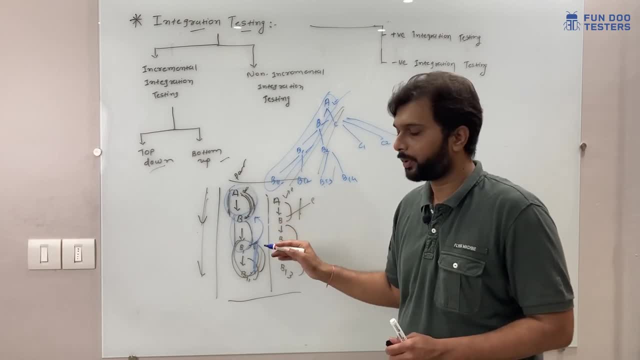 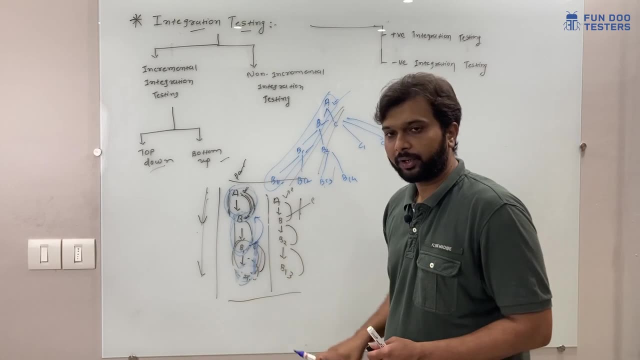 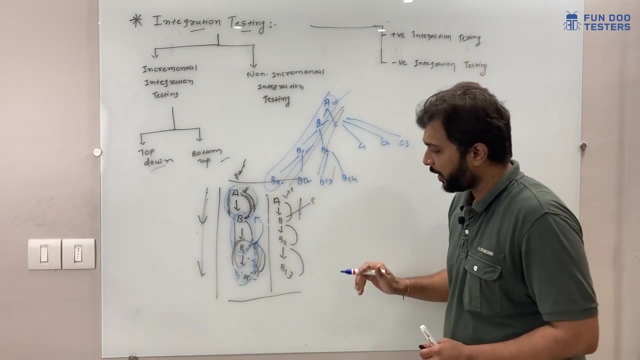 So we can have these two modules and we can perform the top down later. or if we are going to test B2B1.. In that case we are not worry about the B11.. We can easily test the data flow between these two. But in bottom up, whenever we are going to test from B1, from child to, 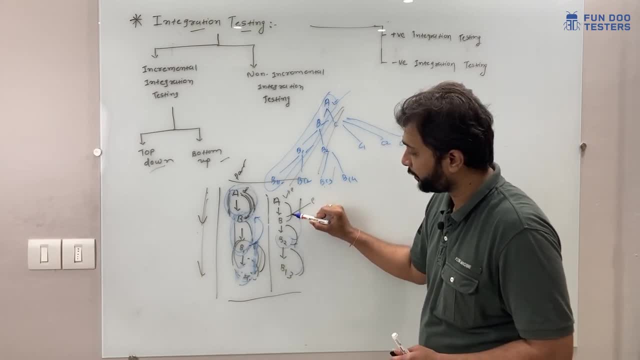 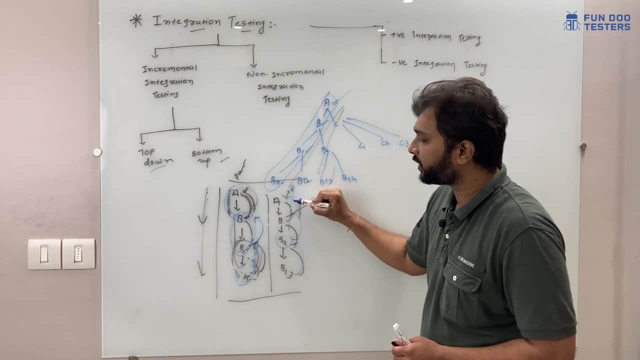 parent B2.. So B2 Is also parent of someone, then B1 also as parent. So in that case, when we are going to test from child to parent, B2.. If we are going to test from B, let's. So in that case each and every parent's module should have ready. 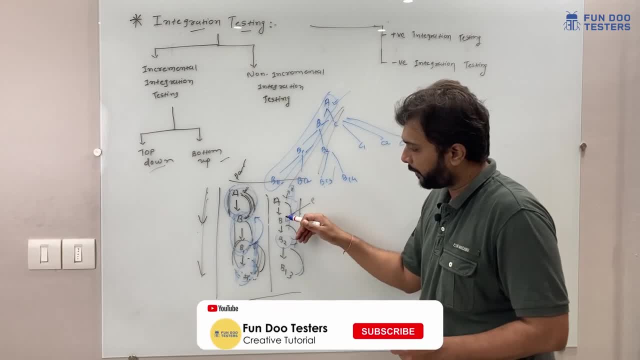 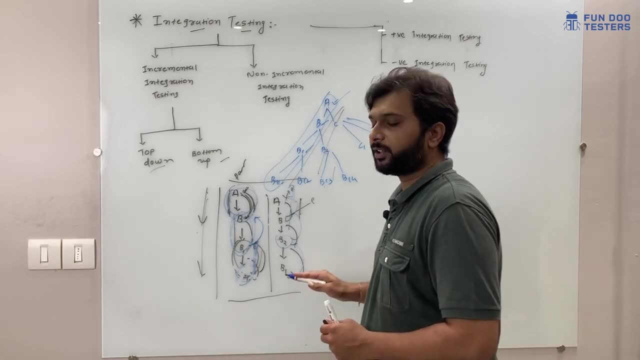 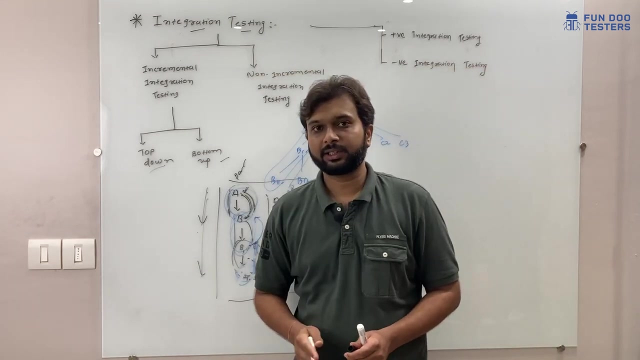 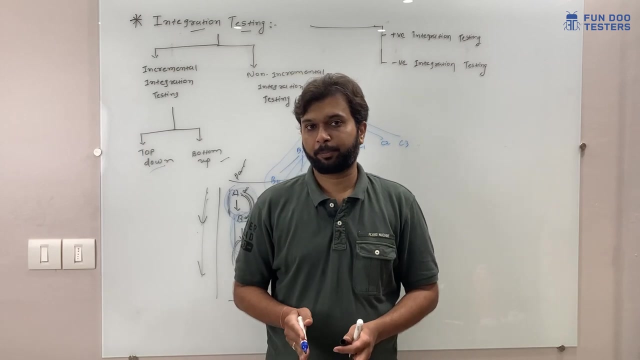 So if parent modules are not ready, then we cannot start from the bottom. This is the disadvantages of the bottom-up approach. Now we understood incremental integration testing. So what is a non-incremental integration testing? Now, whenever we have complex product and we cannot identify the hierarchy, 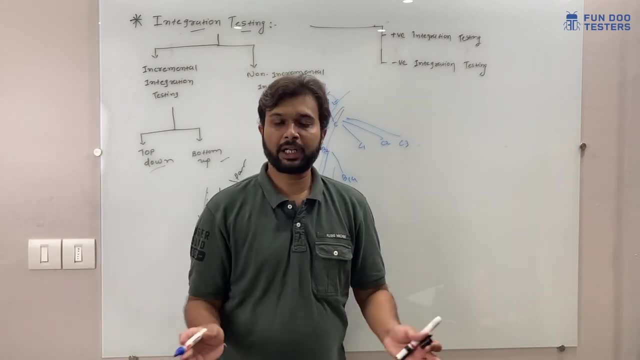 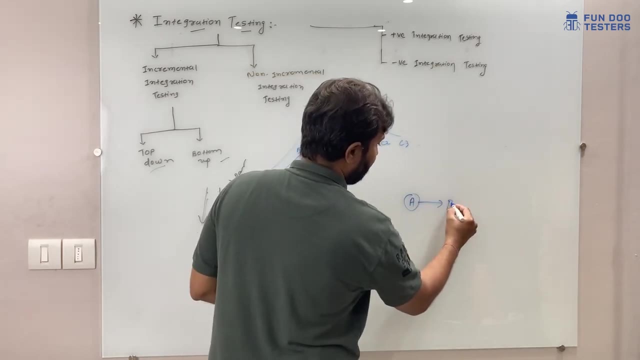 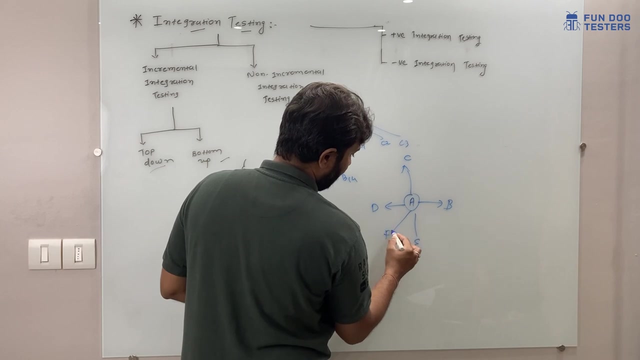 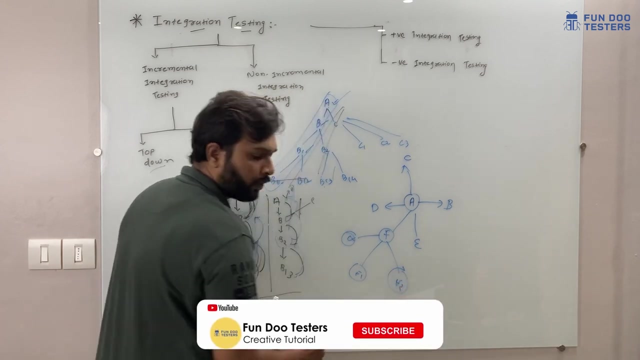 or one module is integrated with the multiple modules. Let's take an example. We have module A and it is integrated with the B, C, D, E, F, F is integrated with the G, F1. F2. That is not a particular manner. 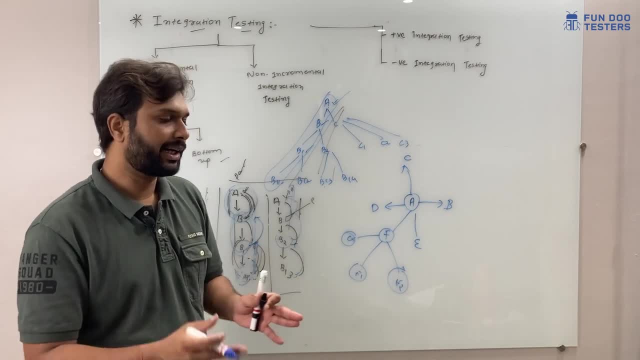 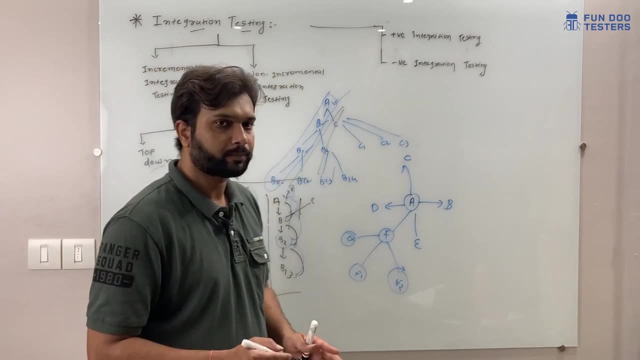 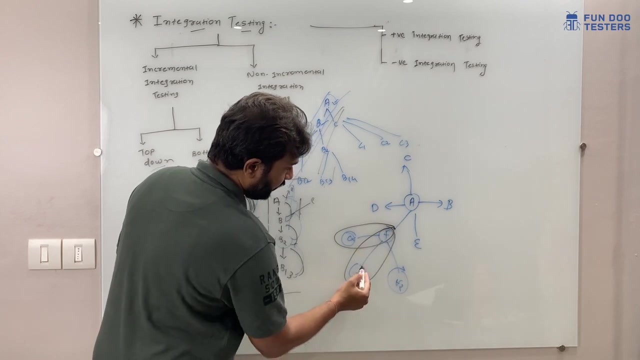 It is randomly connected with all the modules are randomly connected with each other. In that case we have to go with the non-incremental integration testing. We have to test integration flow between the F and G, Then F and F1, F and F2.. 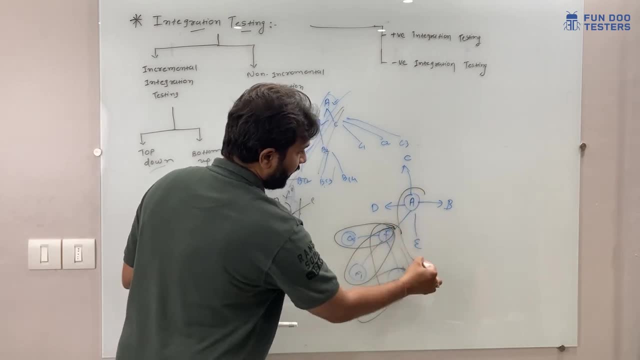 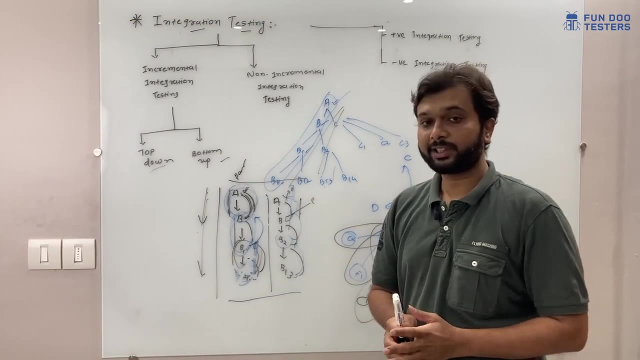 Here there will be a few modules, So we have to test this. A and E, A and B. We have to make different. We have to make different permutations and combinations. The biggest drawback of non-incremental testing is we can miss few integrations. 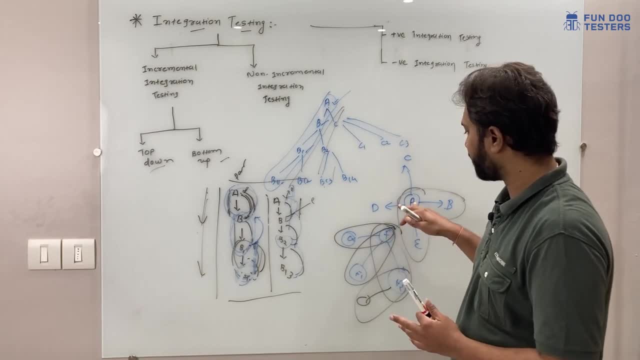 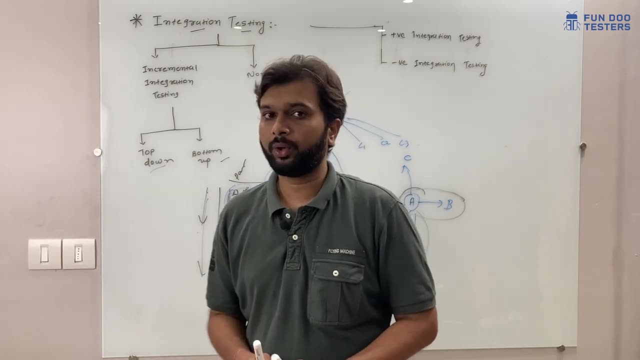 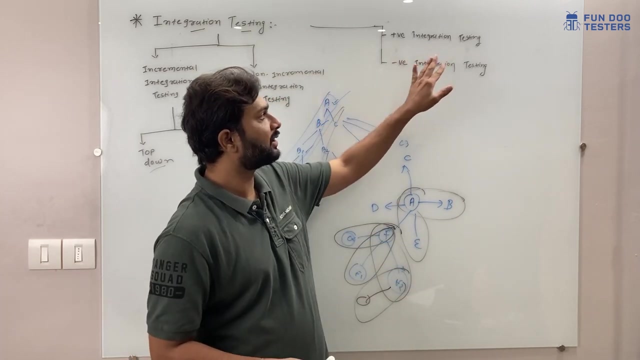 For example, there are complex integrations There can be a chance of- if we can miss data, integration flow between the A and D. This is the biggest disadvantage of the non-incremental testing. Now we can differentiate integration testing into another term which is called positive integration testing and negative integration testing. 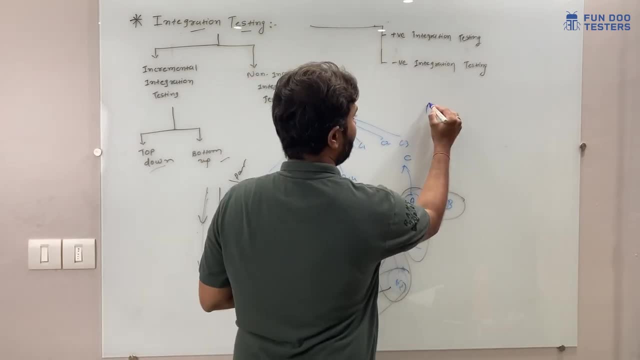 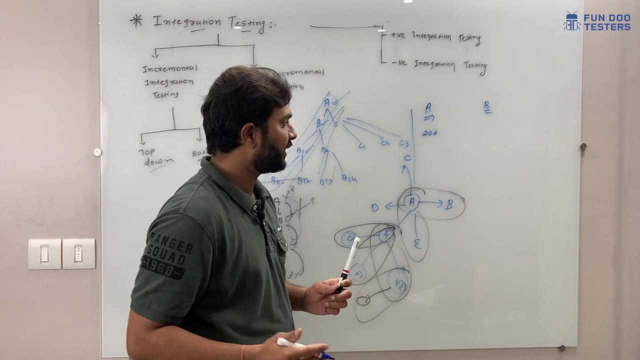 In this case what will happen? For example, let's say person A wants to send money to person B. Now we understood in earlier, we understood the wallet scenario. So in the same case, let's say person A is sending 200 bucks to person B. 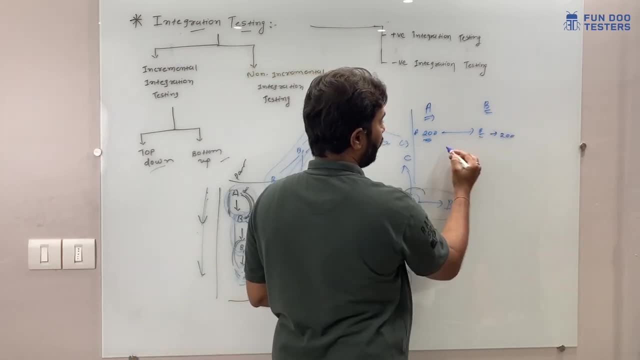 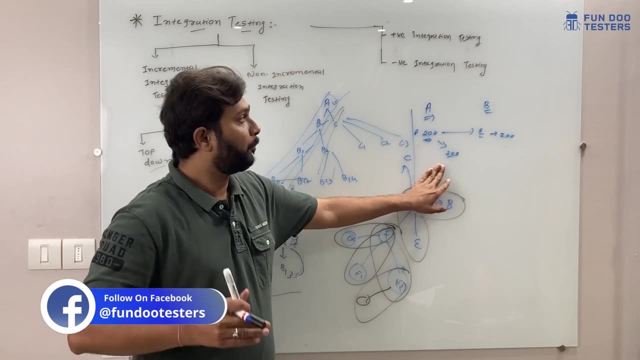 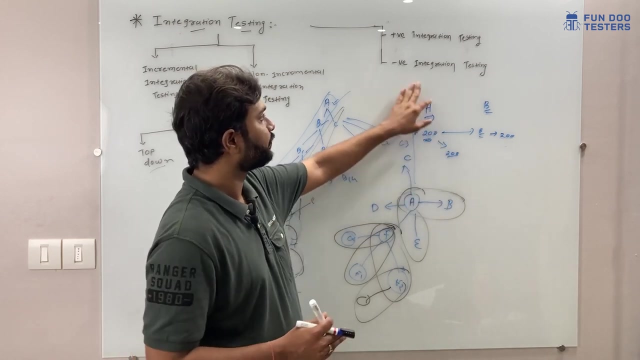 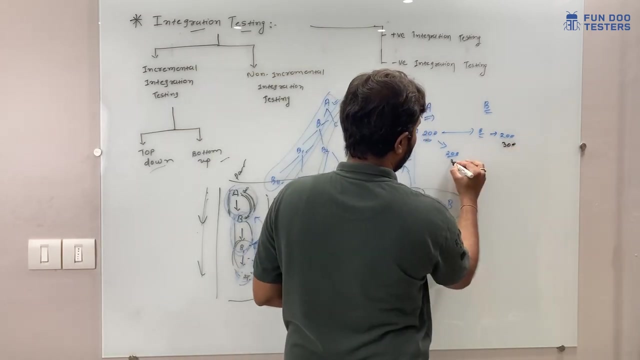 We have to test person B has received 200 or 200 is deducted from the bank account or wallet. This is called positive integration testing. Now, what we can do, We are going to test in negative integration testing. Let's say, person A has sent 200 bucks but person B has received 300, or here it is deducted 300 or 100 rupees. 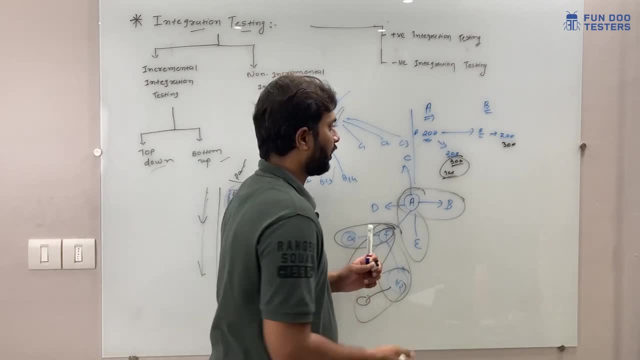 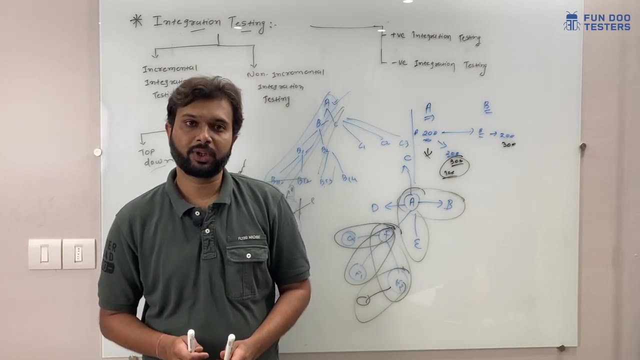 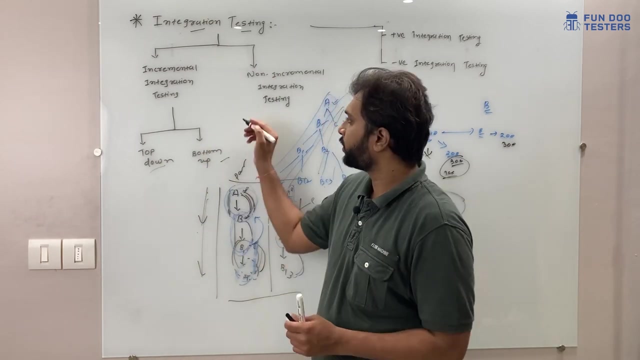 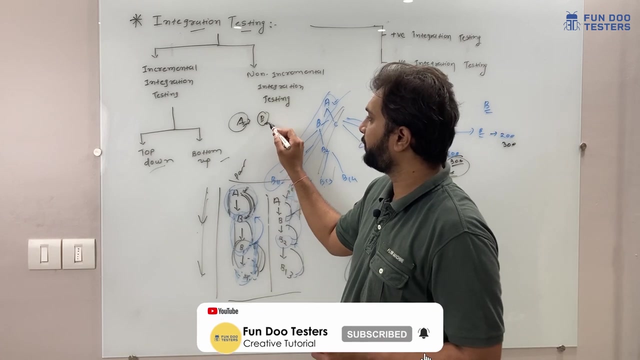 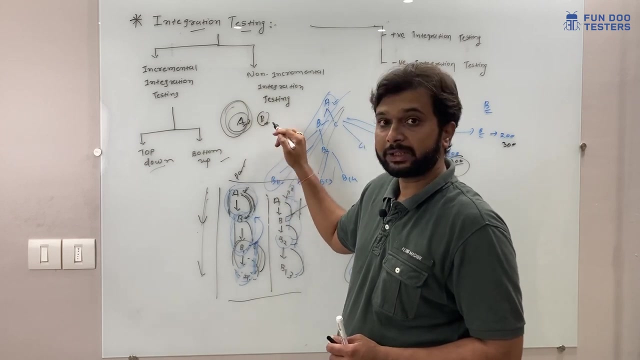 So we are going to verify that it has not deducted some other account instead of 200. So this is called negative integration testing. Now a very important question comes: If we are going to test data, If we are going to test the data flow between the two modules, module A and module B, but module A is not available or module B is not available, and I want to test that if module A is working or not and module B is costing more. 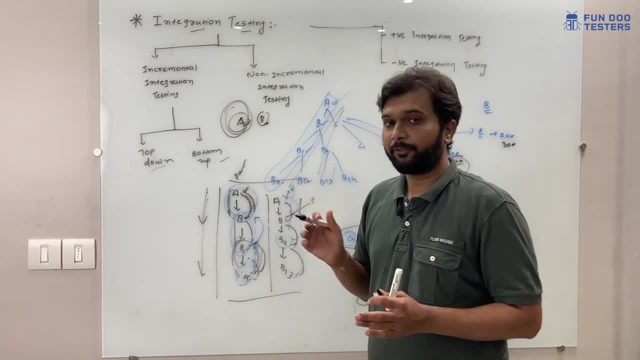 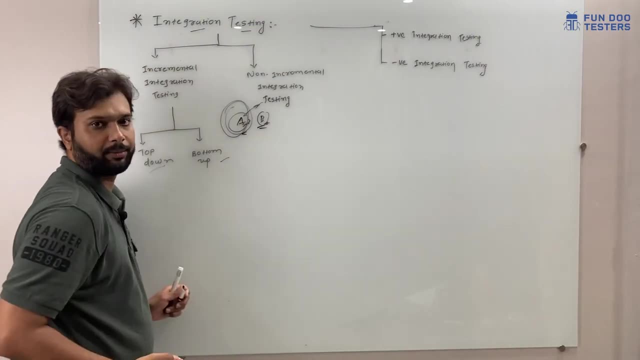 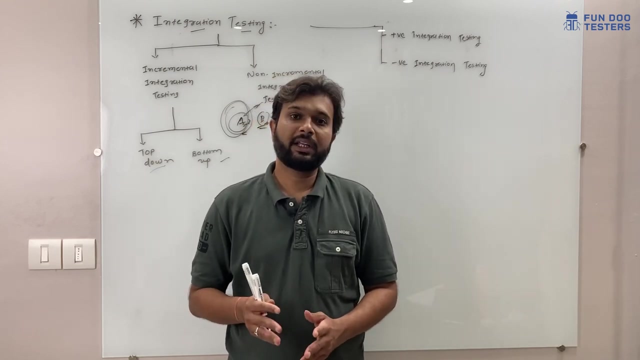 If module B is costing more, then first somehow I have to validate module A is working or not. Let's say module B is not available in industry or in real time Whenever we are testing- If we are going to test banking application or wallet application- we cannot integrate our test wallets with the real time bank account. Otherwise, we are running with the huge money or we need huge amount in our bank account, And many companies are outsourcing the tester or outsourcing the developer. They can steal the money or they cannot count all the money. So in that case, what they can do instead of integrating with the real bank? 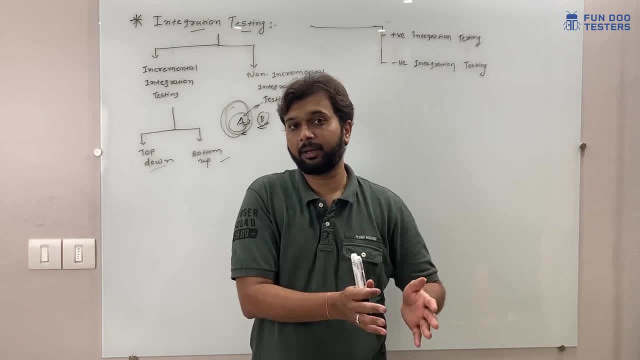 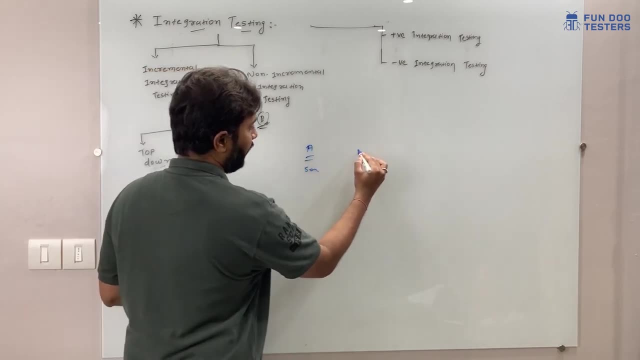 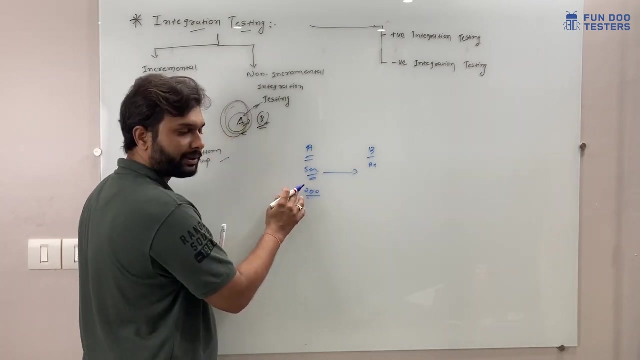 They will integrate With the dummy dummy they can, they will create the dummy module and they will test the data flow. So let's say I have wallet A sender and wallet B receiver. If person A wants to send money- 200 bucks- in that case person A should have linked bank account. 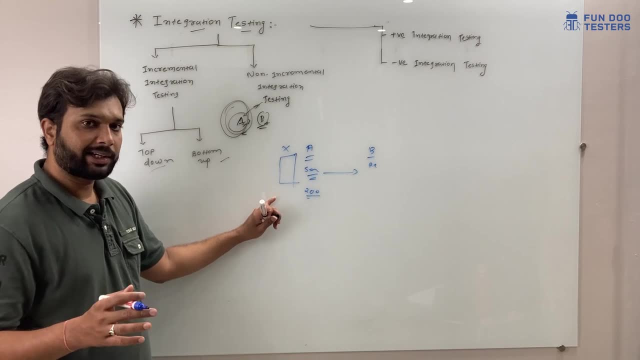 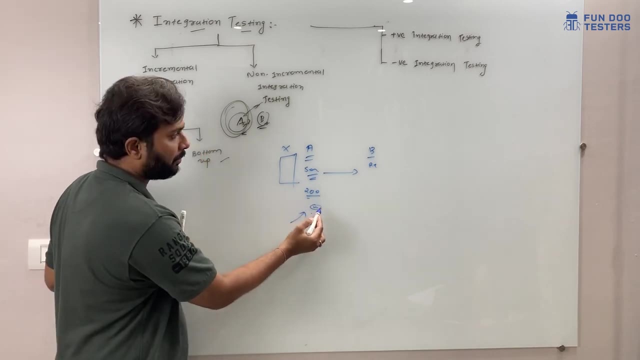 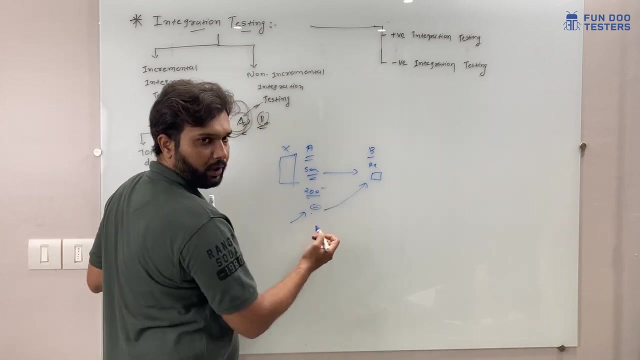 But I don't want to use real bank account. So what, in that case? what I can do, I can whenever I'm going to send money. by that time I will send some acknowledgement Message and this guy will receive some acknowledge message from the bank or from the wallet. 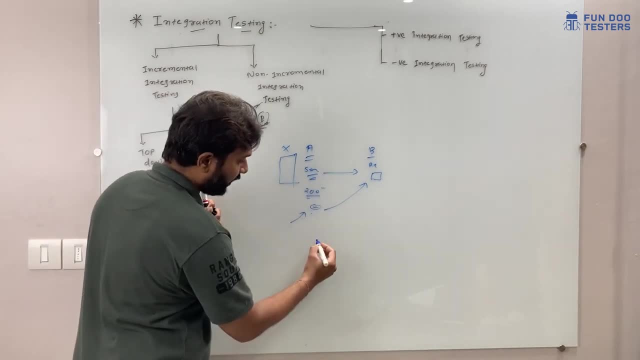 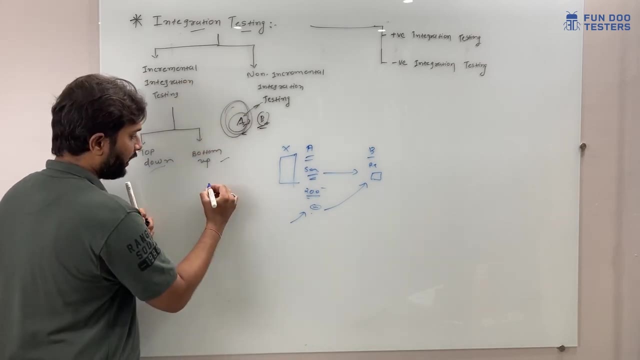 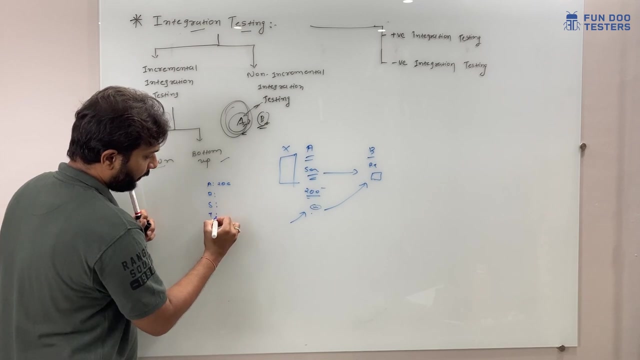 So, internally, what will happen whenever I'm going to send the money? So it will have the user details, For example, let's say it is, it is a data file and it is the amount detail, 200, receiver detail, sender detail. then a few token. 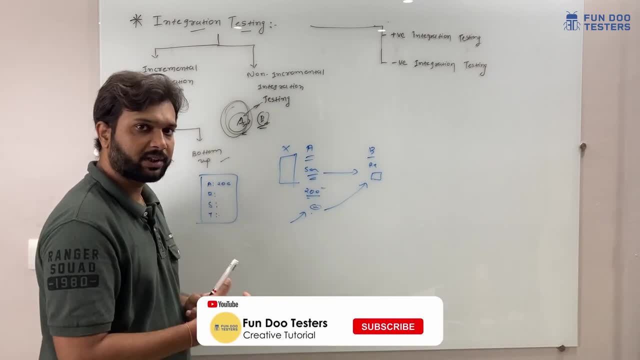 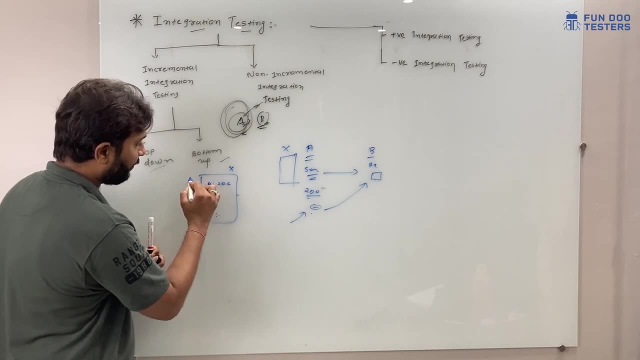 So in that file I am sending- Actually I'm sending- the data They. it will be a packet, So I know to validate with the bank. instead of validating with the bank, I will create some random module and whenever that particular module will receive this data it has to receive by the bank. 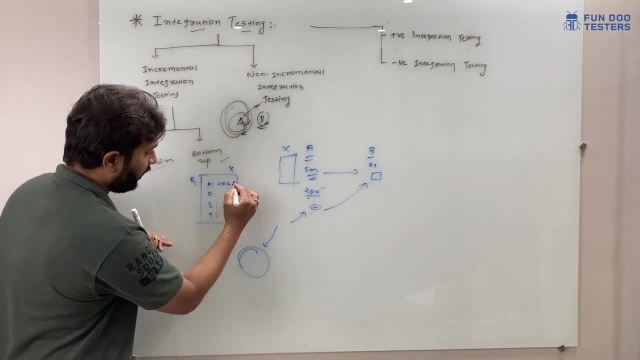 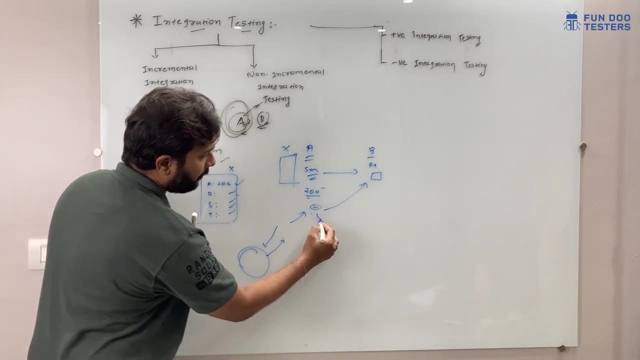 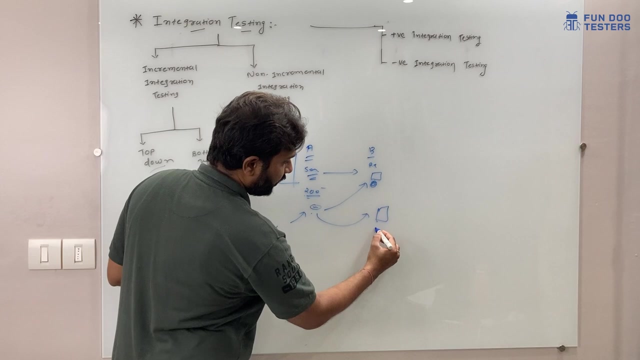 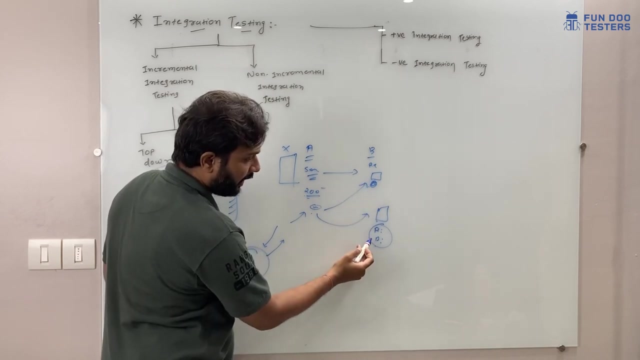 Instead of: I will send to this model and this will verify if there is a for data available or not. If this for data is available, then he will send OK and amount will transfer to the B user. B also will receive One simple packet with the receiver name amount. once the receiver receives this packet, they will send back OK or not OK to sender. 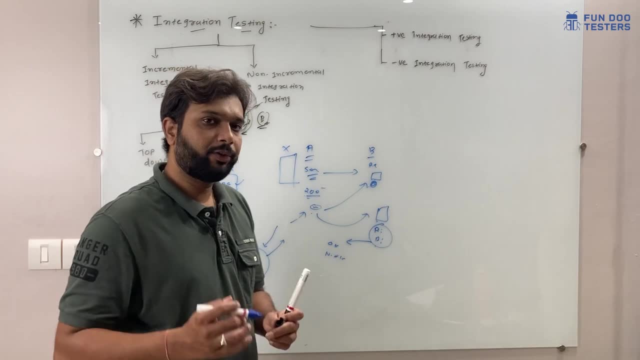 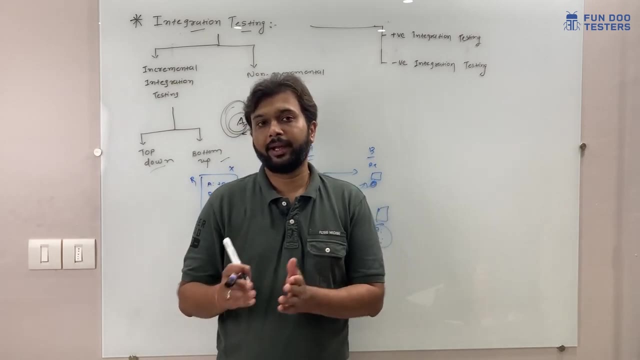 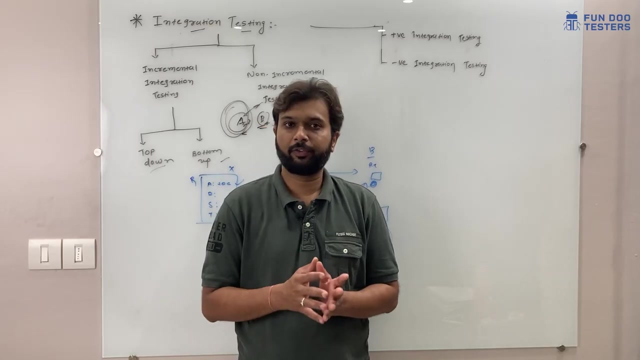 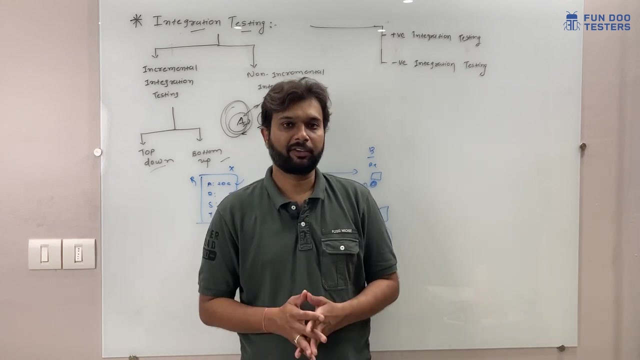 So this is how they can create a dummy module. So whenever we don't have a module ready by the time, we can create a dummy module and that is called as a stub and driver flow. please note it down: Definition. So whenever we don't have a real time modules and we want to test the integration, in that case we can use stop and driver flow. 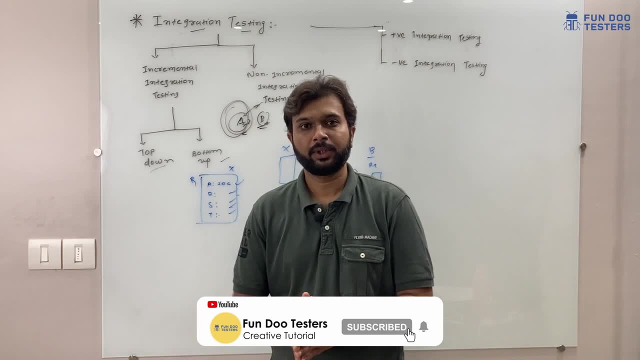 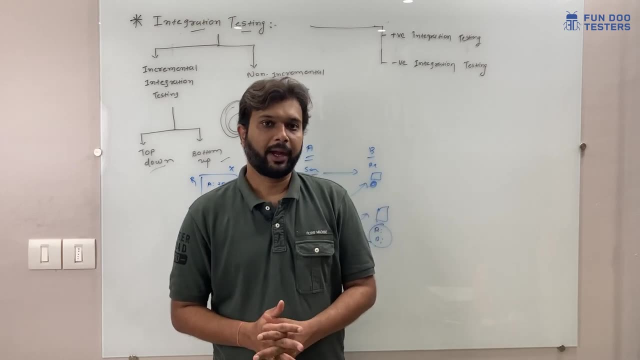 So I hope everything is clear. If you have any doubt in any types or how to do the integration testing, you can ask in the comments section. I will be happy to answer. if you- and please don't forget to say it- or like this video, and please share this video with your friends. Thank you so much. We'll see you in the next video.